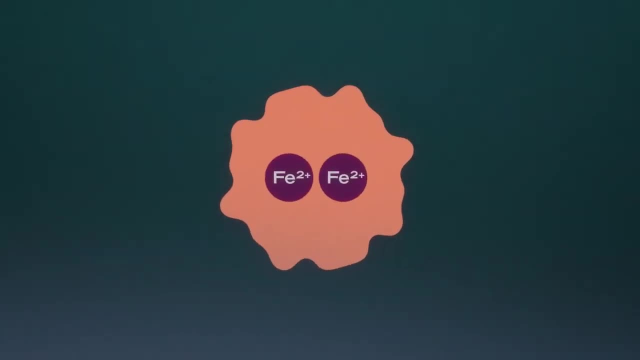 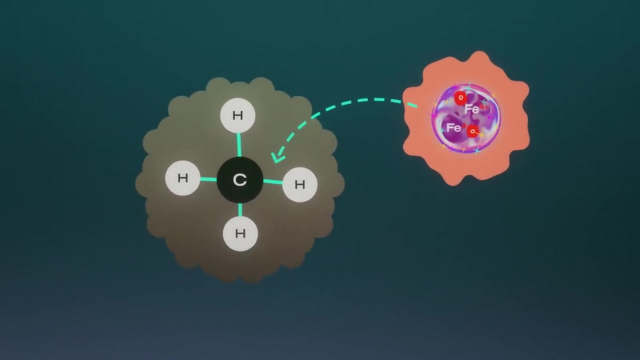 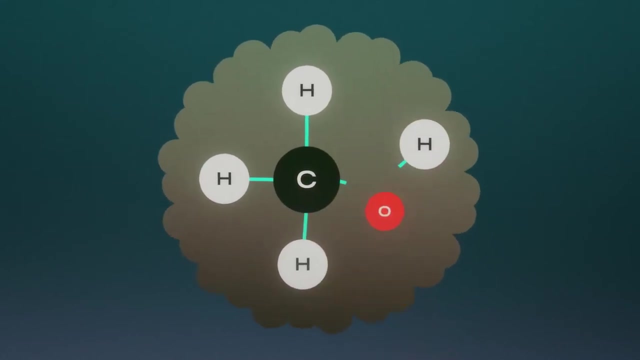 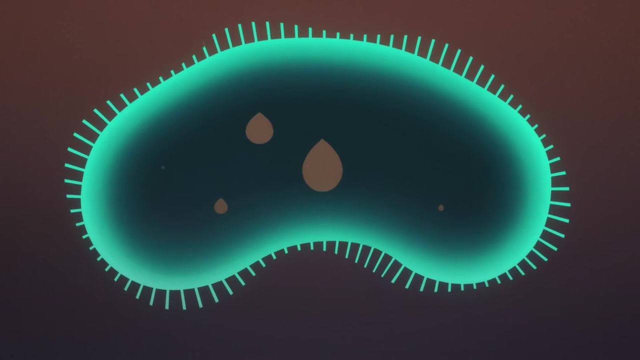 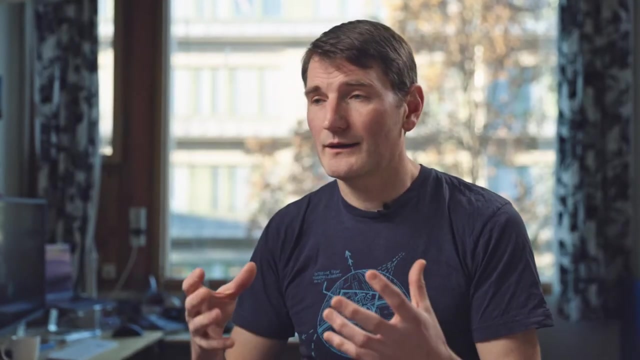 succeed in acting like one strain of bacteria which contains a protein so ingenious that it can hold two iron atoms and let them become so reactive, so highly charged, that together they form an almost nuclear- And this is something that we would really like to be able to do- Then we could take this very 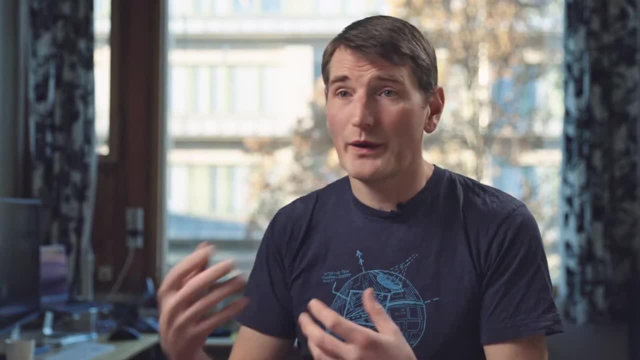 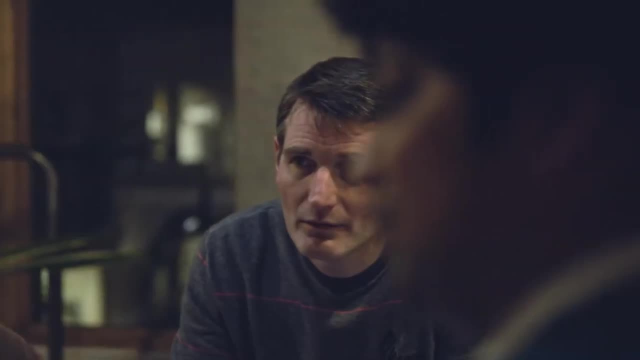 potent greenhouse gas and transform it into something useful like biomass or fuel, And this is something that we would really like to be able to do. Then we could take this very potent greenhouse gas and transform it into something useful like biomass or fuel, But so far no one knows how the bacterium does this. It is an extremely difficult mystery to solve. 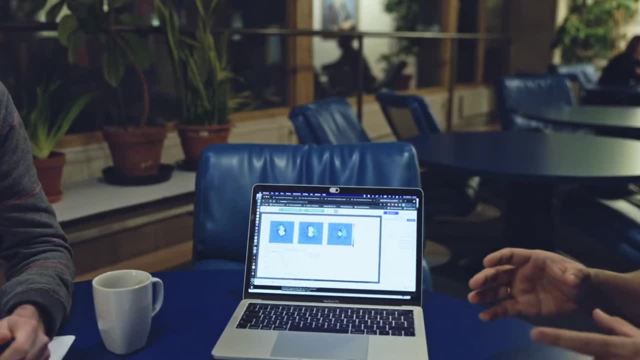 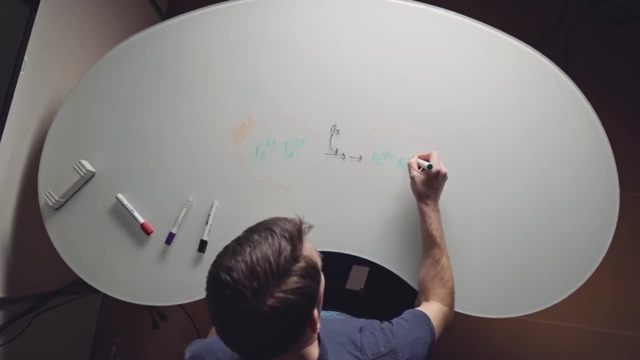 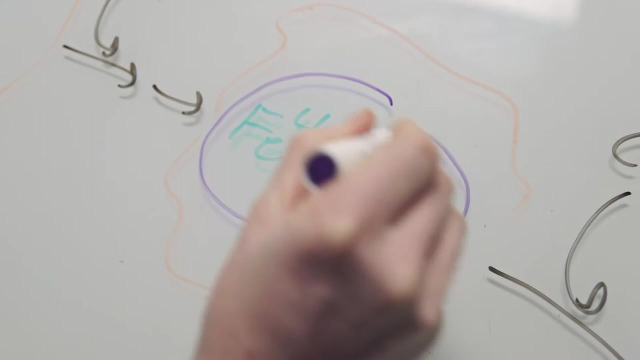 how the bacteria's protein manages to hold on to and control that magical sphere. To reveal this, Martin wants to take pictures of how it works. Yes, and this is actually really difficult, because these iron ions, or the magic sphere, if you'd like to call it like that, they are so highly charged. so they become very reactive but also really unstable. So as soon as you're exposed to any kind of radiation to take a picture, you lose that state. So that's the challenge of this whole thing: to be able to take a picture while they still have the properties that are required to do the chemistry. 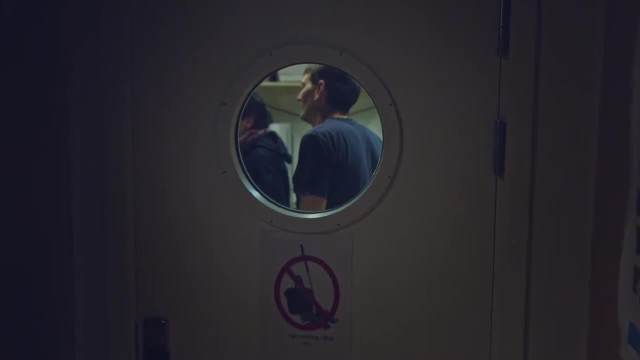 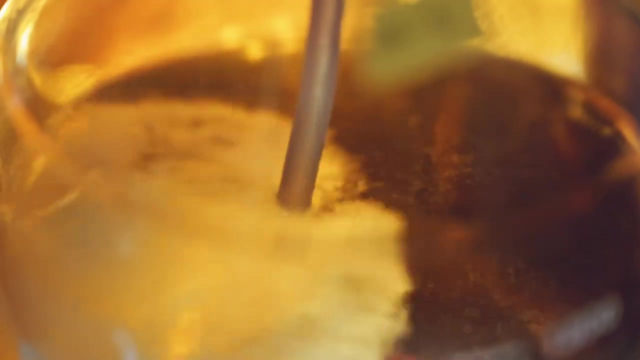 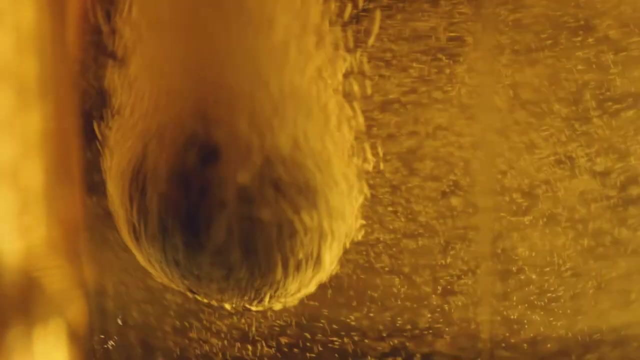 In order to do this, Martin and the team start by developing the bacteria's ingenious protein, the one that will hold the sphere. A massive amount of bacteria is therefore grown in this liquid. The bacteria are then crushed and, after a series of purification steps, the desired protein has been separated out. 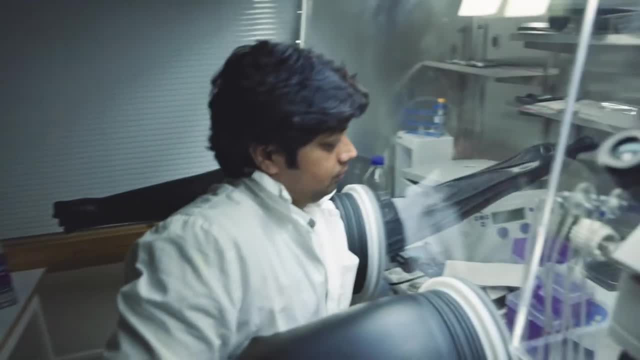 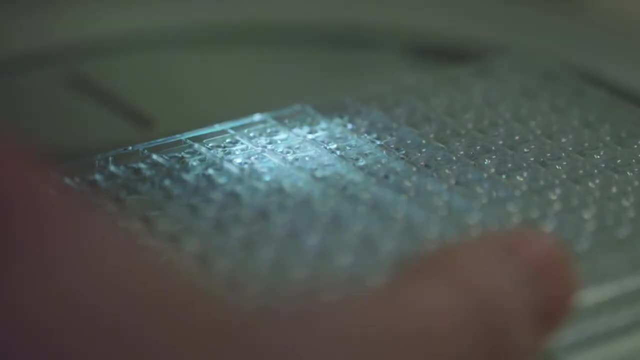 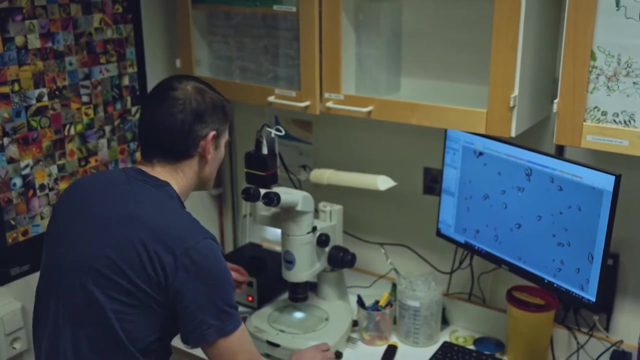 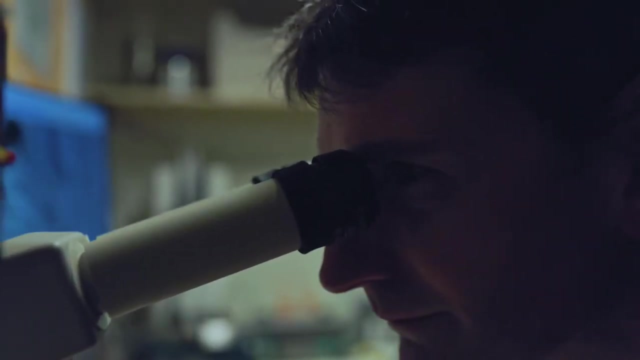 But in order to be able to take the pictures, the protein must first be formed into crystals, Then a radical machine is needed to take the pictures, while the protein crystal is still holding on to that magical sphere. And with this step Martin has had a little luck, because a few years ago, 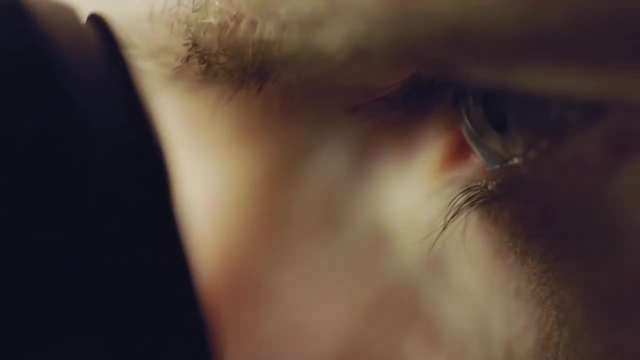 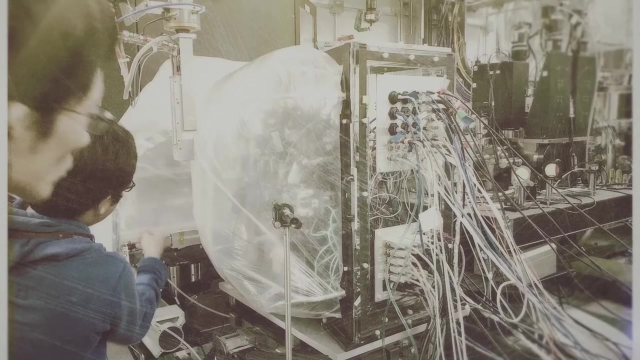 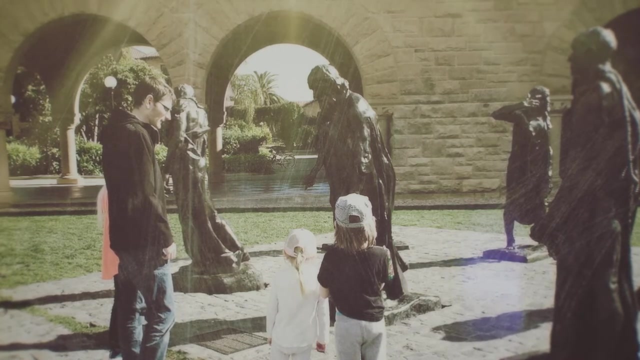 he was a visiting professor at Stanford University in California. Yeah, I mean, this is an amazing opportunity to have as a researcher to go to see new places and talk to other scientists and discuss new projects. And, of course, California is not a bad place to live with, you know, San Francisco. 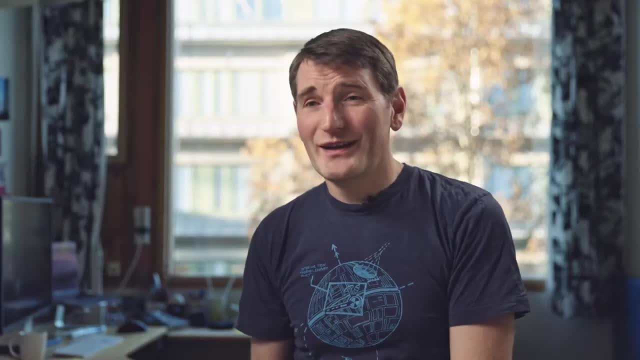 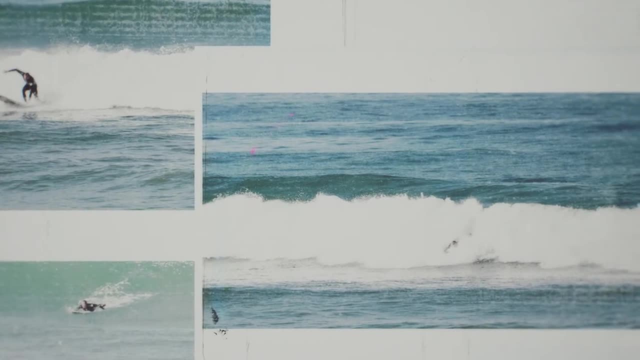 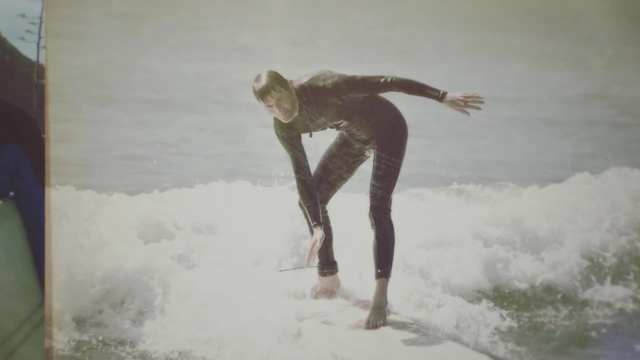 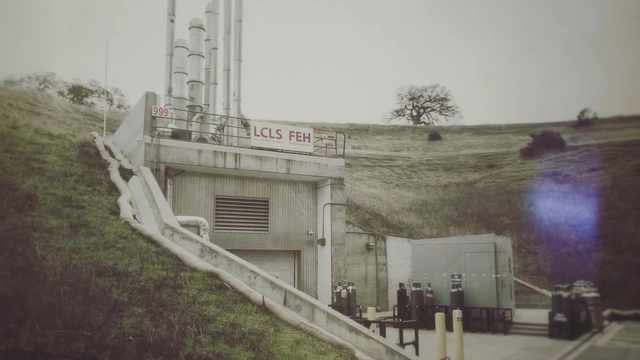 national parks and surfing. My surfing skills are really really poor, but I like them to be better. and, perhaps most important of all, at stanford, martin found his dream machine so big that it filled an entire cavern. wow, yeah, this machine. it sends out x-ray laser pulses. 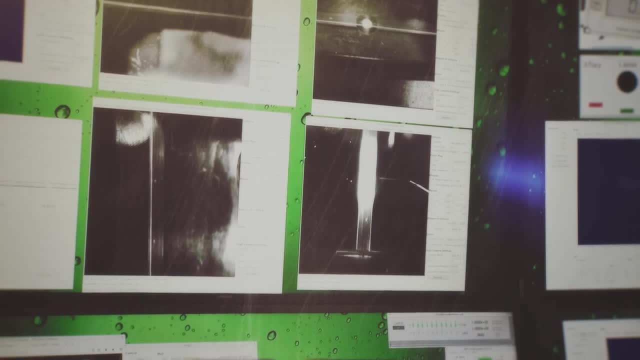 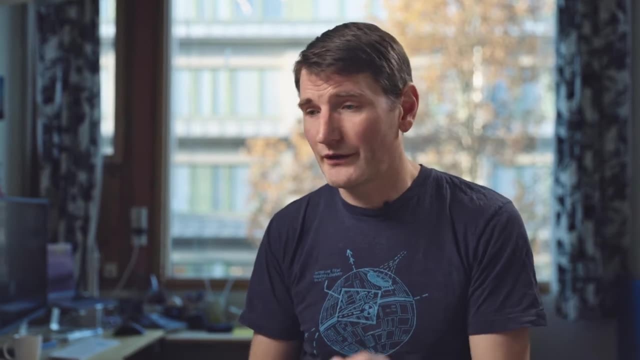 that are so incredibly short: a few femto seconds, that's a millions of a billions of a second. uh, you know, light travel seven times around the globe in one second, but these light pulses are only a few micrometers, or thousands of a millimeter long. at the same time, the energy density is so high. 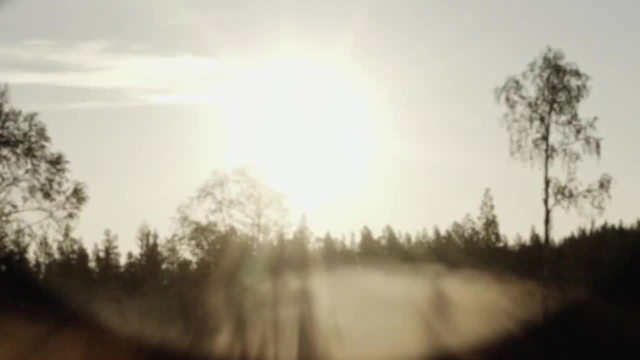 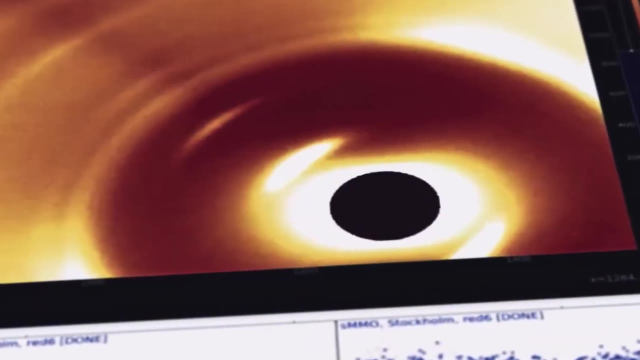 that it would be the equivalent of focusing all of the sun's light energy that hits the earth down to one square millimeter. it's really amazing. and then i realized that this machine could really help us to take this picture of this magic sphere that we haven't been able to do. 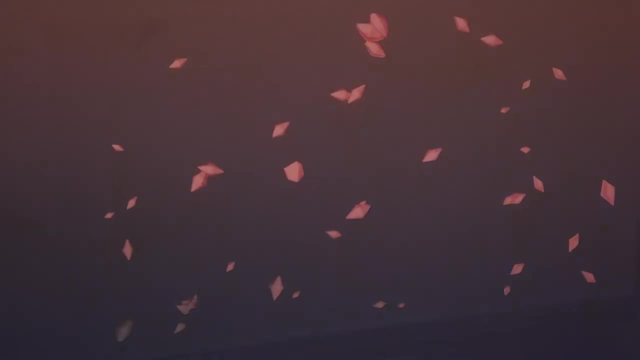 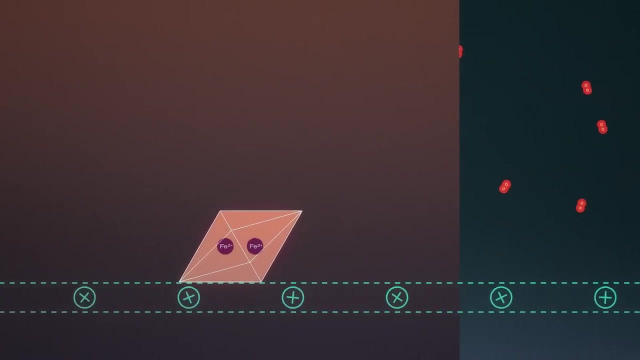 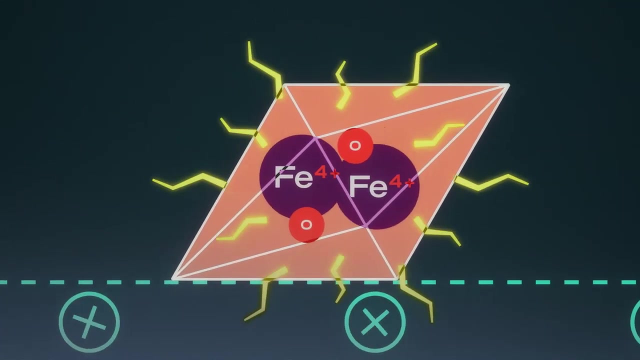 the crystals with the bacteria's protein must therefore travel from stockholm to california. here the protein crystals are placed on a small conveyor belt. there oxygen is added, which reacts with the iron atoms, which then becomes charged with increased power, creating that magic sphere. and then the crystals of protein. 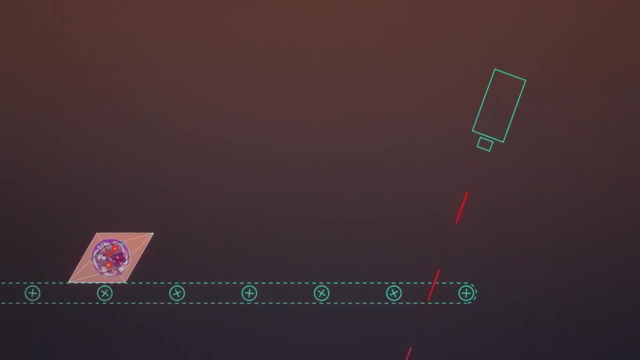 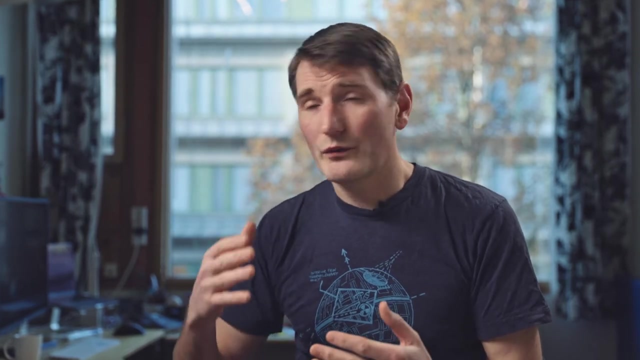 atoms and all go in to be x-rayed to get their picture taken. and when this happens, there is so much energy that the crystal explodes. yes, we blow up the sample, but the nice thing is that that doesn't matter because the pulses are so short, so we get the picture before the sample has the time to blow up. so that's the. that's the neat. 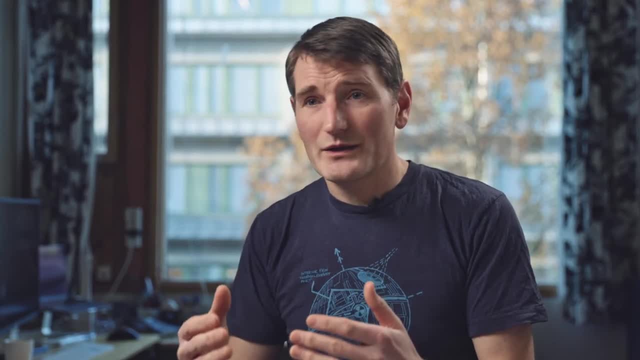 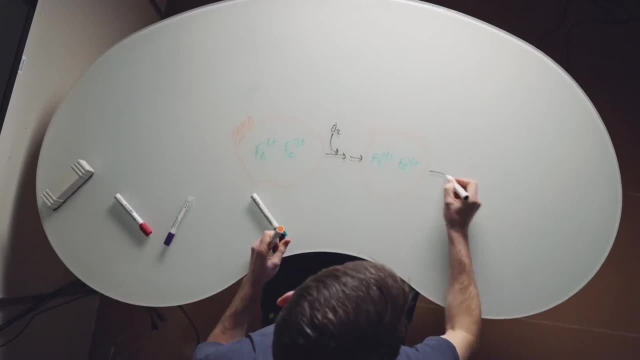 thing and stuff that is so sensitive that we can't touch it, that we blow up, and so far he has successfully managed to take pictures at slightly lower energy levels. this one, for example, is really interesting because it shows how the protein is just set up to start. 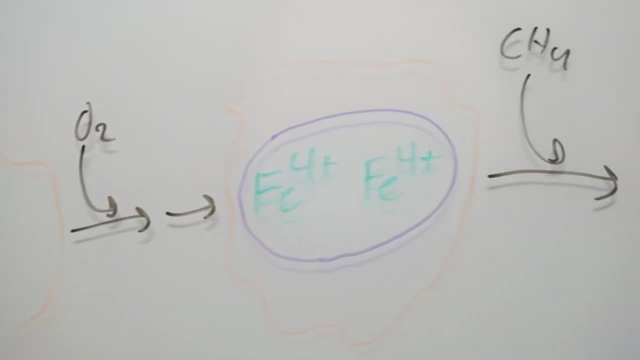 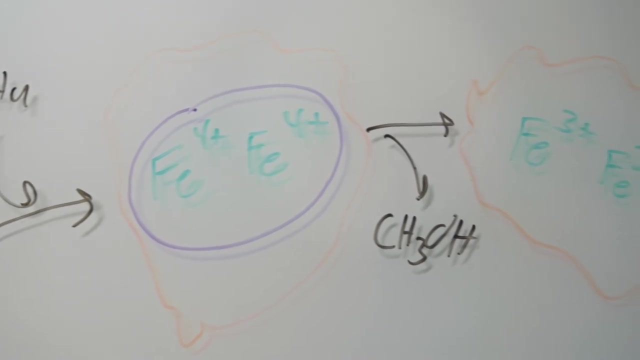 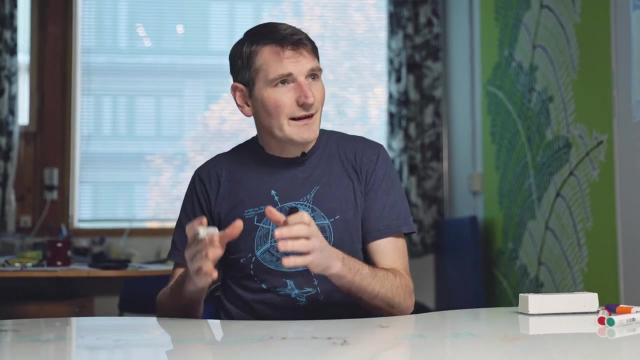 to react with oxygen to to start the entire reaction. now it's just a matter of getting that picture at the precise instant when the magic sphere is caught, and right now we're putting all our efforts into to getting pictures of these fully charged states that are required to do.